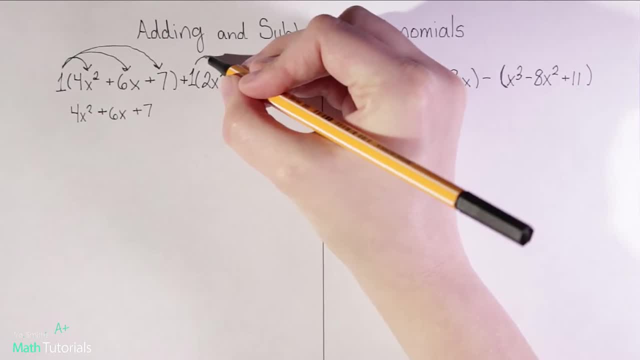 a set of parentheses around it, And what that means is there's an understood positive one in front of those parentheses that needs to be distributed to get rid of the outside parentheses- parentheses. So we'll do the same thing again. Positive one times positive. two x squared is 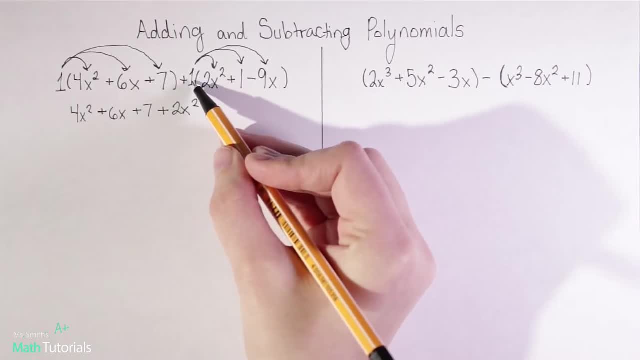 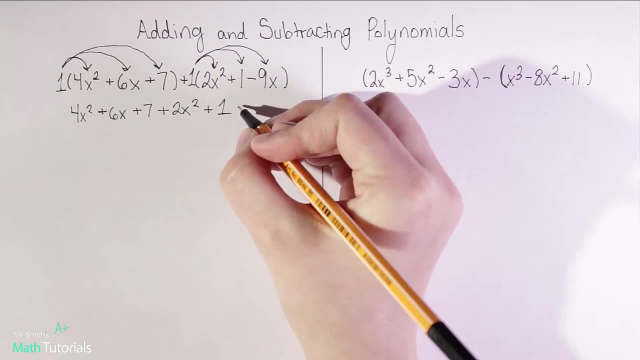 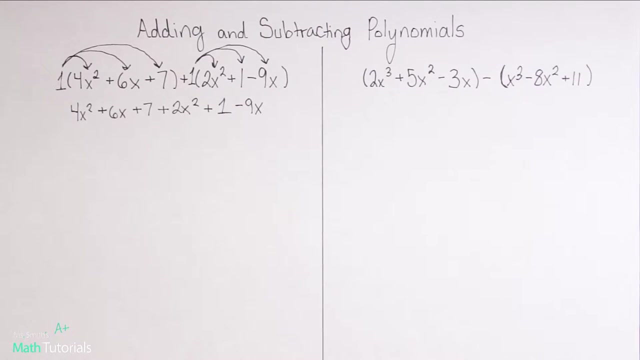 positive. two x squared Positive one times one is positive one Positive one times negative. nine x is negative, nine x. So a lot of teachers skip over that step and they say, okay, just you're adding, so just get rid of the parentheses and combine like terms And there's. there's nothing wrong with that. 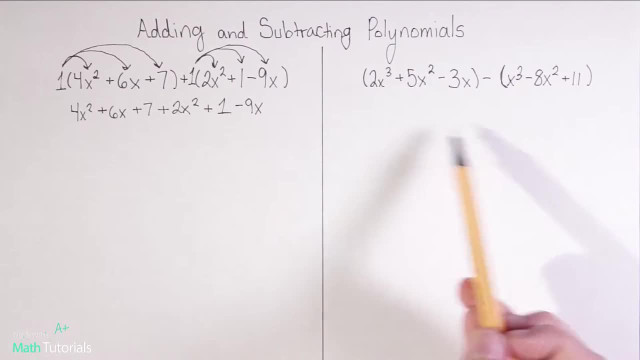 but, as you'll see when we get over here in a minute, this step of you distributing the one is actually pretty important, Even though when we multiply a positive one times anything, it doesn't change the number. Once we get a negative it will. So that's why I really like to show that step, even 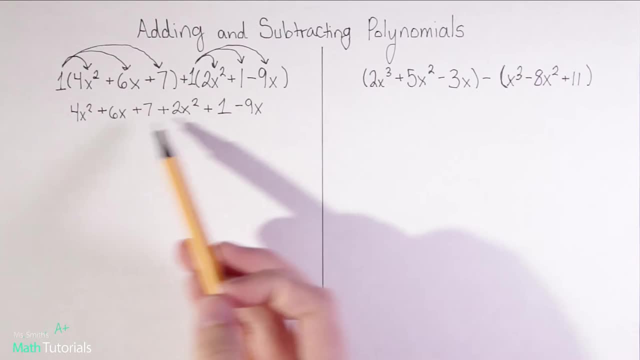 though it seems kind of like, okay, well, we just ended up with the same thing. I think it's. I think it's important to show. So now that we've gotten rid of our parentheses, we need to go ahead and combine any like terms that we have. So I've got a four x. 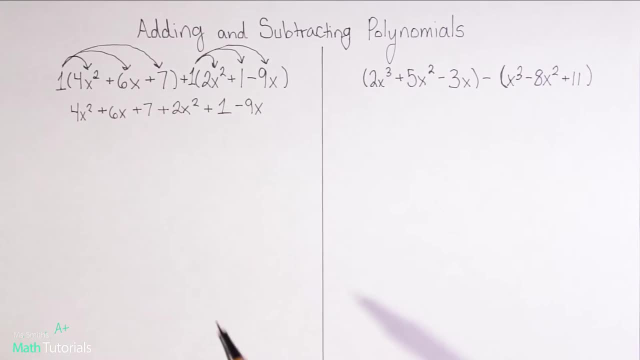 squared here, and then I also see an x squared here. In my last video we talked about combining like terms and that when we're adding or subtracting we have to have the same variable- x and x- and the same exponent, So they both would have to have an exponent. 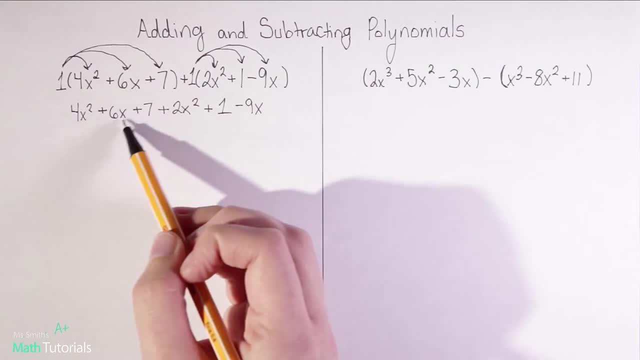 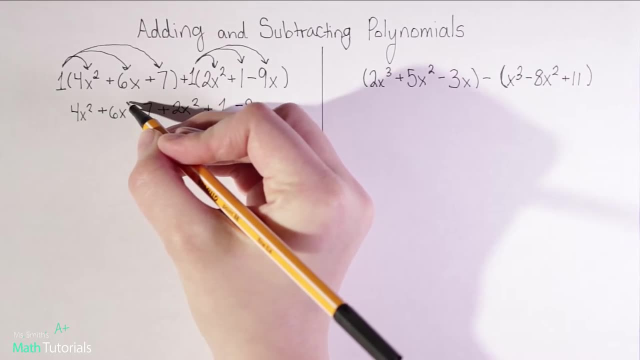 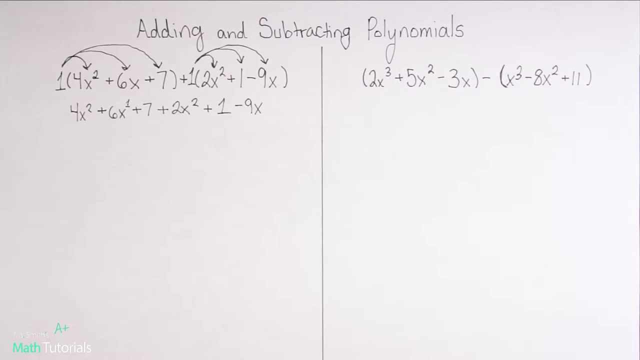 Of two. So I can't combine this four x squared and say this six x. A lot of students will say, oh well, they both have x, But this one has an understood exponent of one, So it's not the same exponent. We can't combine them through adding. So let's, let's combine what we can. So four plus two, Some. 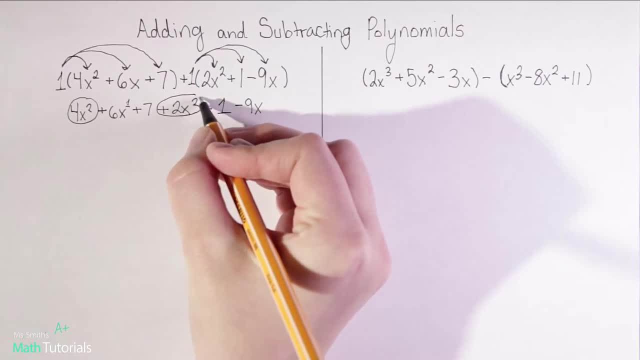 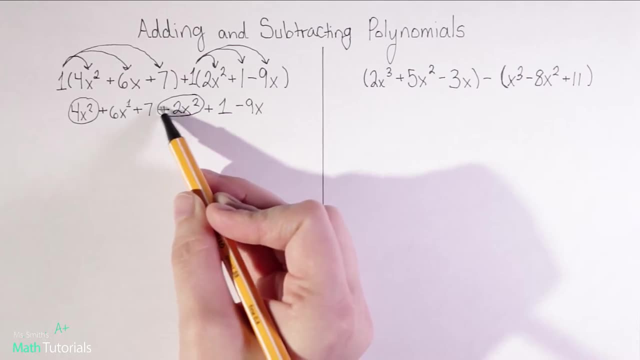 students like to circle what they're combining. If that works for you, please do it. Notice I'm I'm circling the side. You can see here that we have a sign in front of the two x squared as well. That's really important. 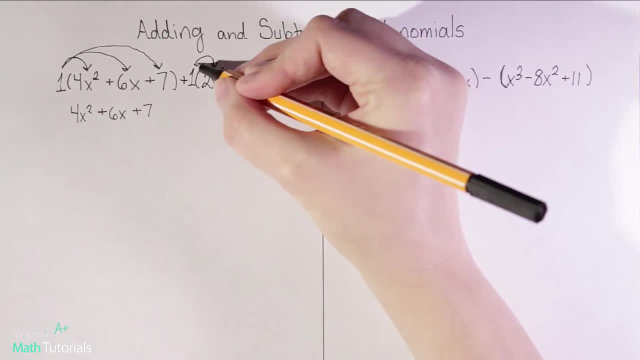 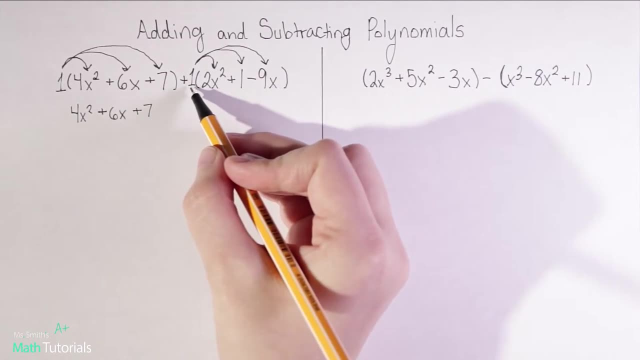 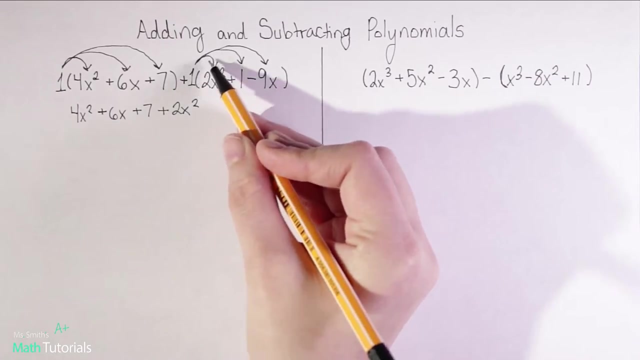 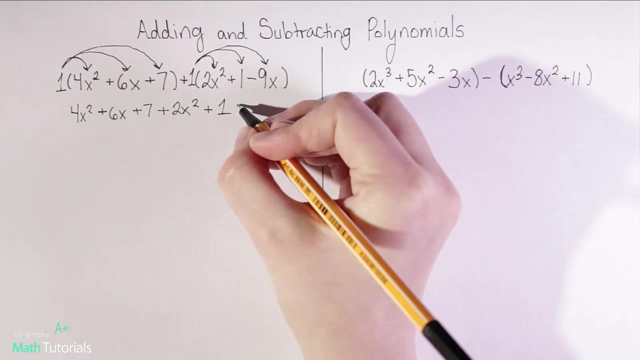 of those parentheses that needs to be distributed to get rid of the outside parentheses. So we'll do the same thing again. Positive one times positive. two x squared is positive. two x squared Positive one times one is positive. one Positive one times negative. nine x is. 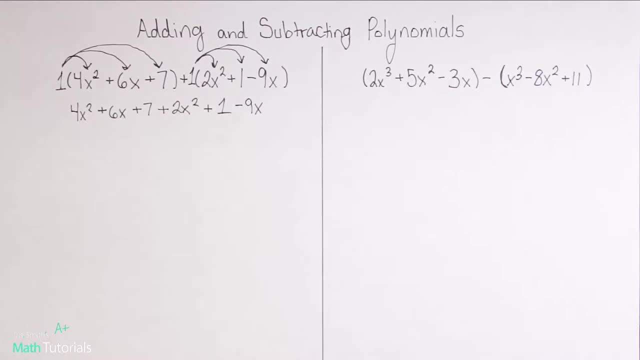 negative nine x. So a lot of teachers skip over that step and they say, OK, just you're adding, So just get rid of the parentheses and combine like terms. There's nothing wrong with that. But as you'll see when we get over here in a minute, this 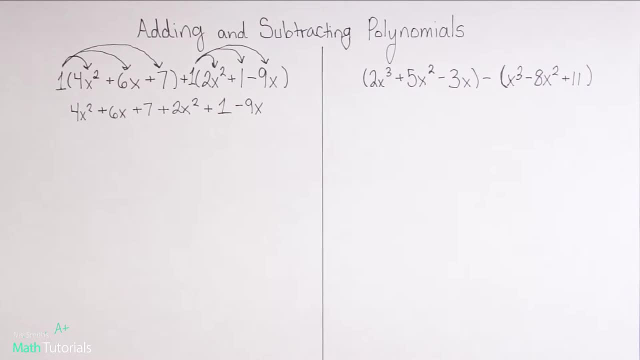 step of you distributing the one is actually pretty important, even though when we multiply a positive one times anything, it doesn't change the number. Once we get a negative it will. So that's why I really like to show that step, even though it seems kind of like. 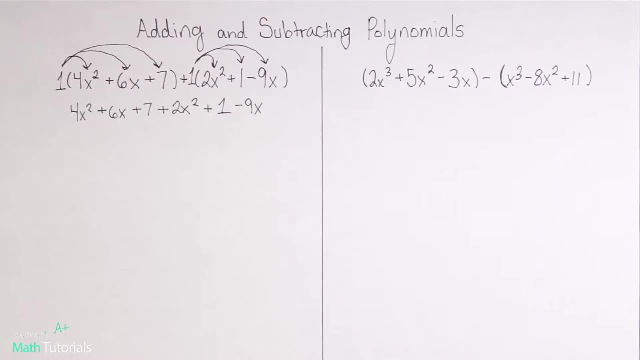 OK, well, we just ended up with the same thing, I think it's. I think it's important to show. So now, Now that we've gotten rid of our parentheses, we need to go ahead and combine any like terms that we have. So I've got a four x squared here, and then I also see an x squared here. 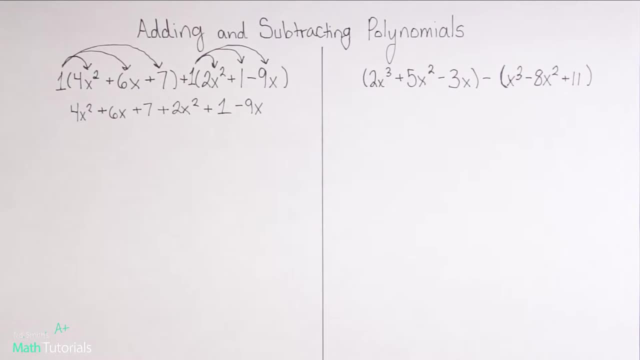 In my last video we talked about combining like terms and that when we're adding or subtracting we have to have the same variable- x and x- and the same exponent, So they both would have to have an exponent of two. So I can't combine this: four x squared and 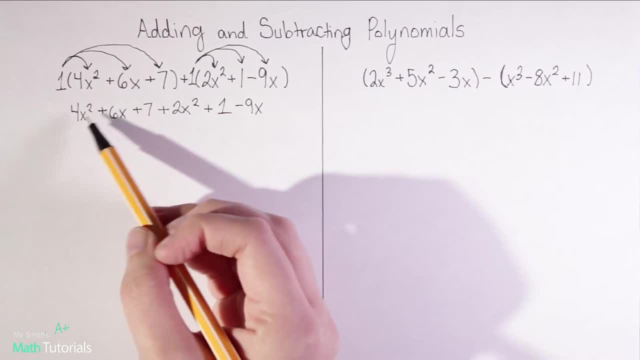 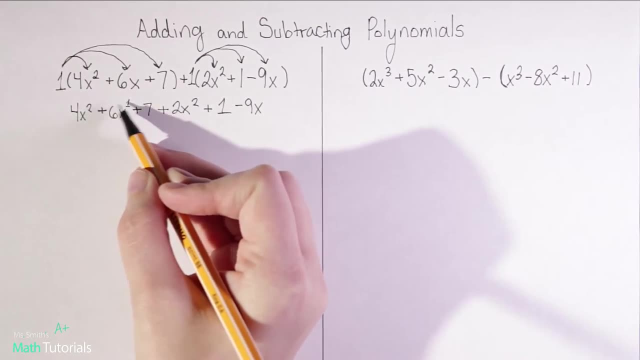 say the six x, A lot of students will say: oh well, they both have x, But this one has an understood exponent of one, So it's not the same exponent. We can't combine them through adding, So let's, let's combine what we can. So four plus two. Some students like to circle. 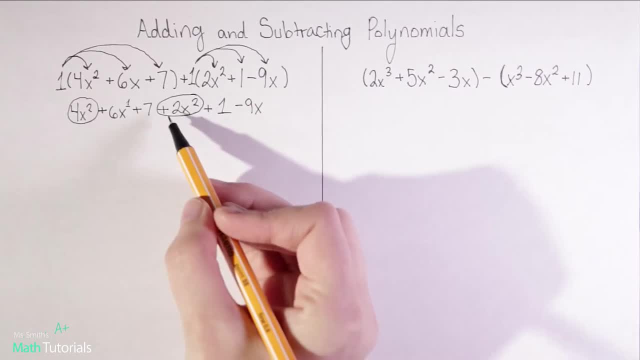 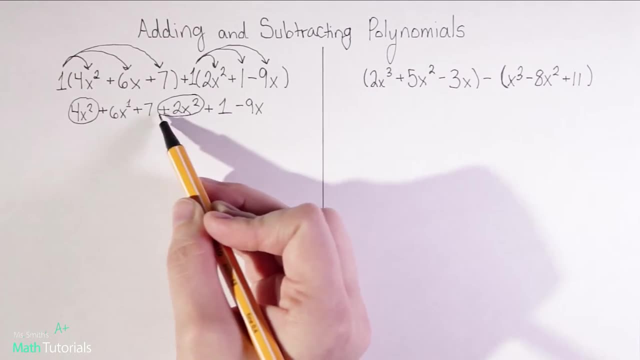 what they're combining. If that works for you, please do it. Notice I'm circling the sign in front of the two x squared as well. That's really important, So I'm going to do that. Well, that's really important because that sign is attached to the two x squared. 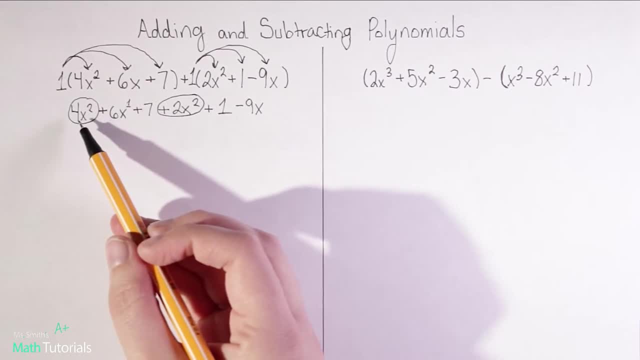 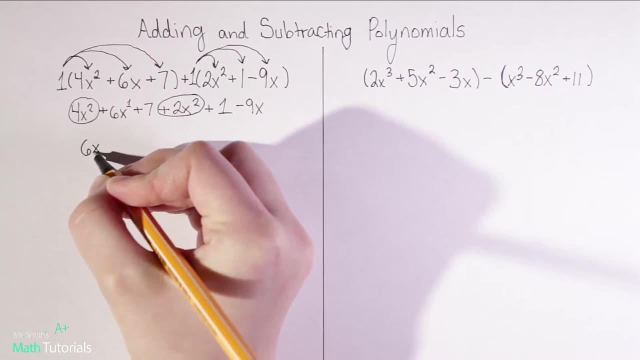 because that sign is attached to the two x squared. Four plus two would be positive six x squared, and x squared stays x squared, So our, when we're adding are subtracting, our variable and exponent stay the exact same. So let's see what else we can combine. I've got a positive six x and a. 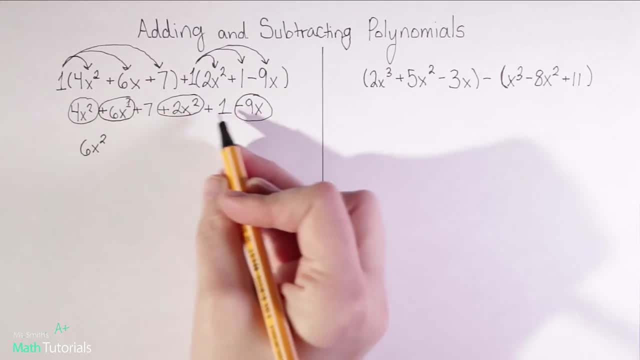 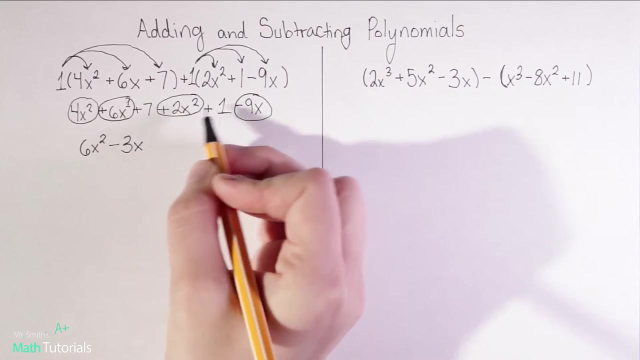 9x. So I can go ahead and combine those two. 6 minus 9 is a negative 3.. So that negative will end up being my subtraction sign, And my variable and exponent stay the exact same. Lastly, to combine, I've got my two constants that I can combine. So 7 plus 1 is positive 8.. So this is: 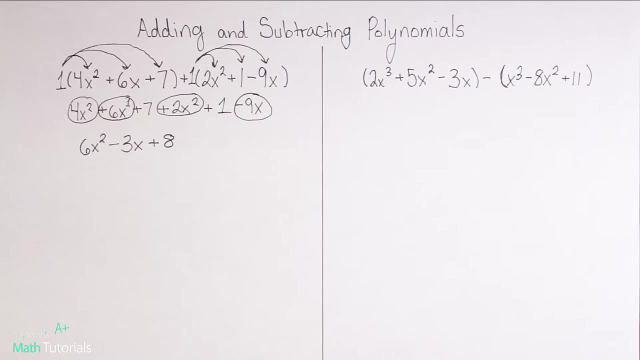 as far as I can take this problem, because I've combined all my like terms. It's important to note that I did write my answer in standard form. So I wrote my highest exponent and then in descending order of exponents, and I have my constant last. So just for fun, just for review. 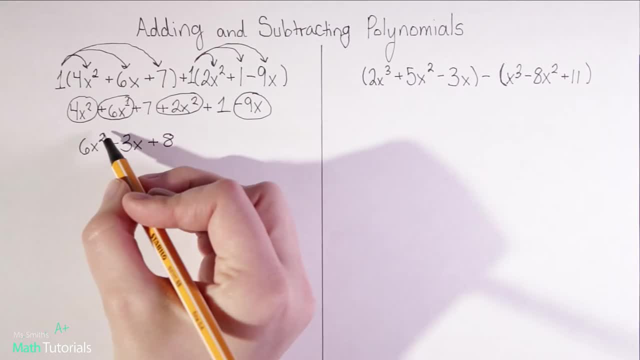 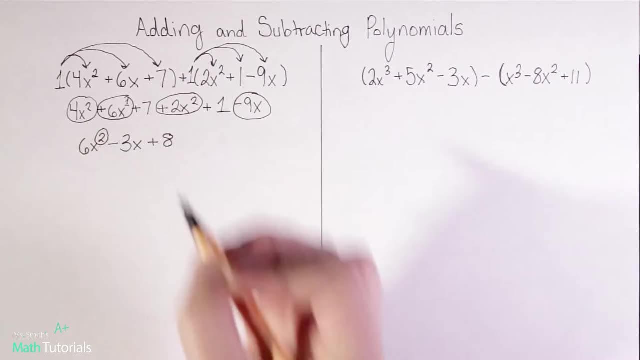 let's go ahead and name this polynomial that we've created. Remember, polynomial names have a first and last name. The first name is based on its degree And then, in this case, we have a degree of 2. So, remember, we call that quadratic. And for its second name, we look at how many terms. 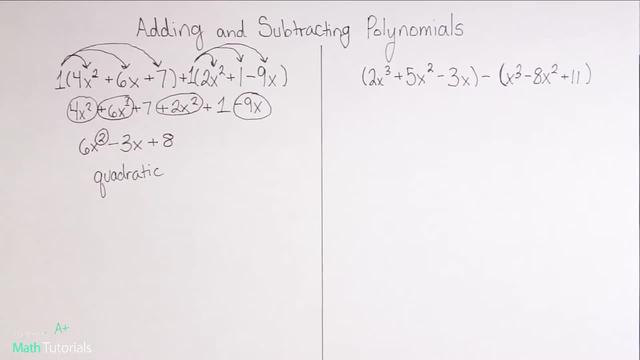 does it have? So how many sections, separated by either an adding or subtracting sign? So in this case, we have 1,, 2,, 3.. So remember, just like a tricycle has three wheels, this is a trinomial. 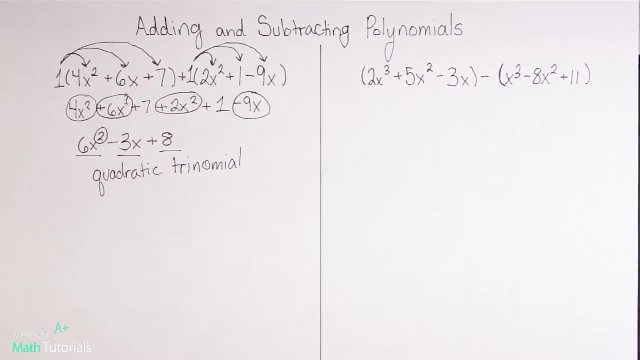 because it has three terms. So that is adding polynomials. Let's look at an example now of subtracting polynomials, because it's a similar concept but a little bit different, In the same way that we had the 1 outside of this parenthesis. 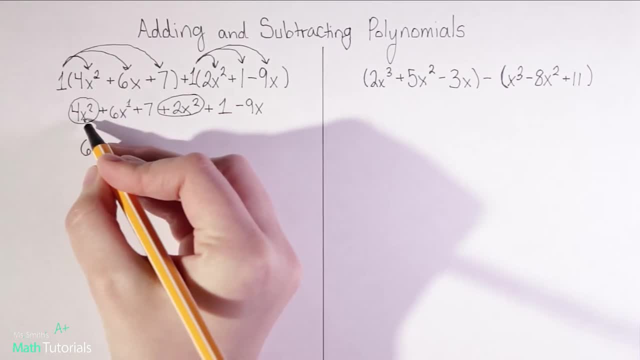 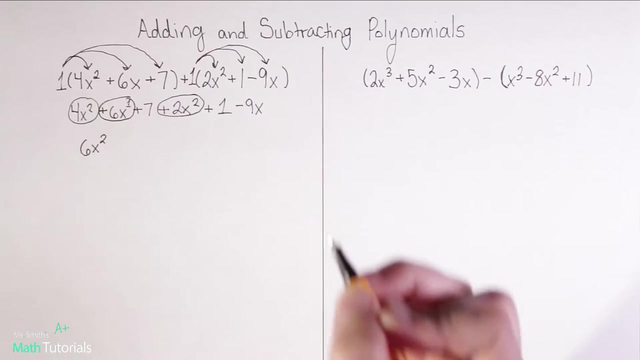 Four plus two would be positive six x squared, and x squared stays x squared, So our, when we're adding or subtracting our variable and exponent stay the exact same. So let's see what else we can combine. I've got a positive six x and a negative nine x, So I can go ahead. 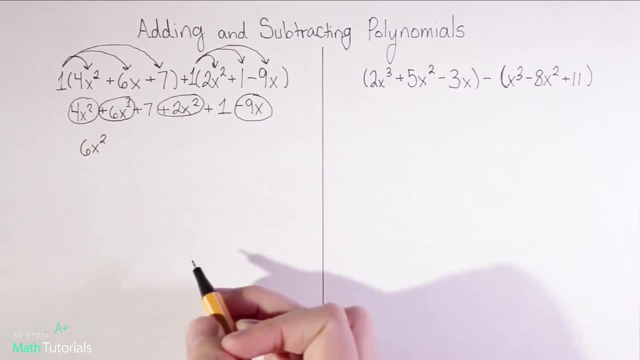 and combine those two. Six minus nine is a negative three. So that negative is will end up being my subtraction sign and my variable and exponent stay the exact same. Lastly, to combine, I've got my two constants that I can combine. So seven plus one is positive eight. So this is as 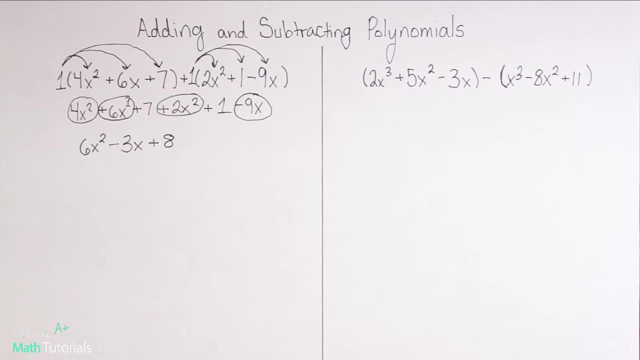 far as I can take this problem, because I've combined all my like terms. It's important to note that I did My answer in standard form, So I wrote my highest exponent and then, in descending order of exponents, and I have my constant last. So just for fun, just for review, let's go. 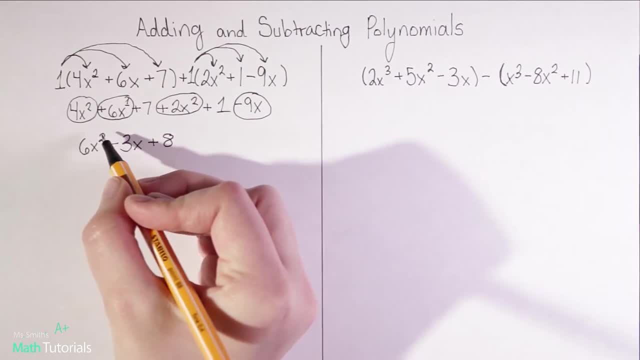 ahead and name this polynomial that we've created. Remember, polynomial names have a first and last name. The first name is based on its degree And then, in this case, we have a degree of two. So remember, we call that quadratic. 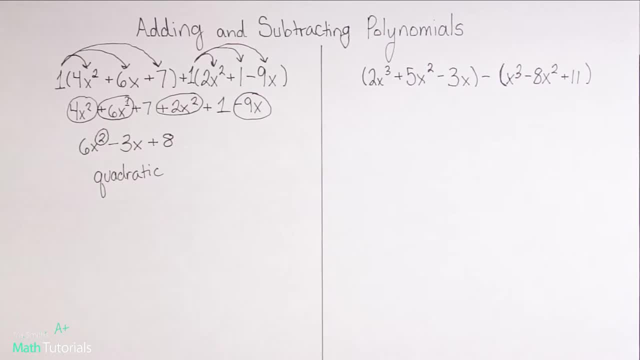 And for its second name we look at how many terms does it have? So how many sections separated by either an adding or subtracting sign? So in this case we have 123.. So remember, just like a tricycle has three wheels, This is a trinomial because it has three terms. So 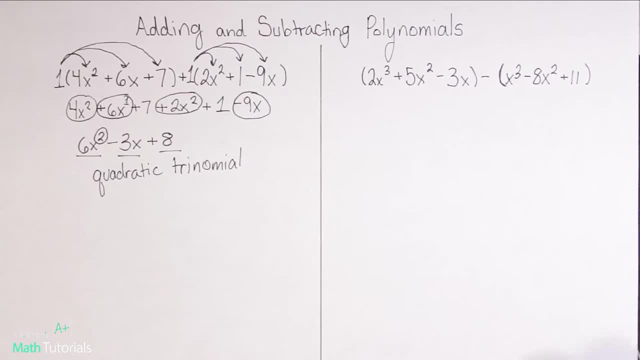 that is, adding polynomials. Let's look at an example now of subtracting polynomials, because this is a concept, but a little bit different. In the same way that we had the one outside of this parentheses, we also would have a one here, So there's a positive one out here. 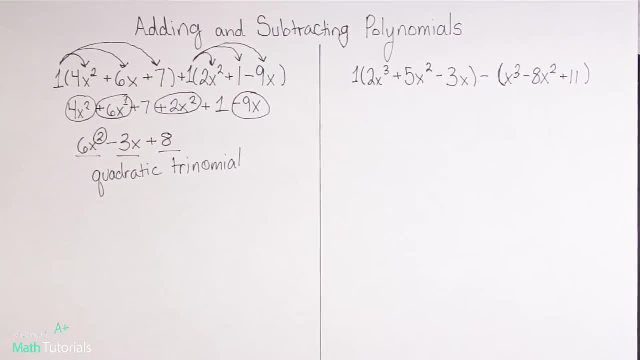 that needs to be distributed throughout this whole problem, throughout this whole parentheses to get rid of the parentheses. So we would distribute this one to every single part of the problem. So one times two x cubed is two x cubed Positive. one times five x squared is positive five x squared and positive one times negative. 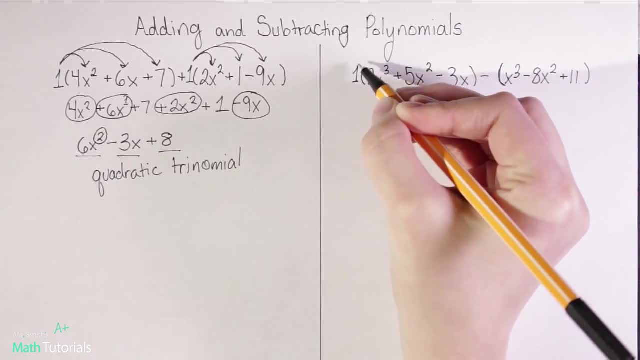 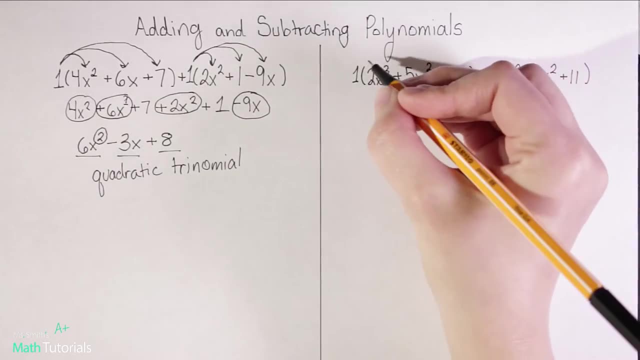 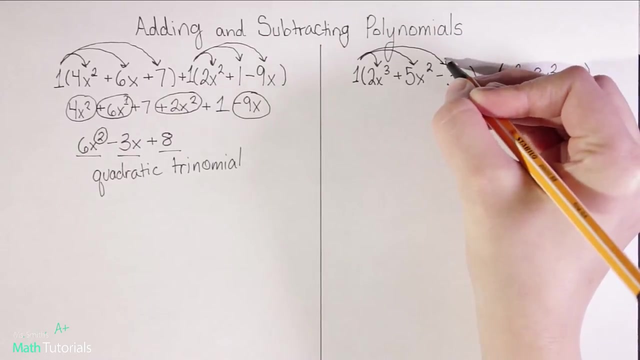 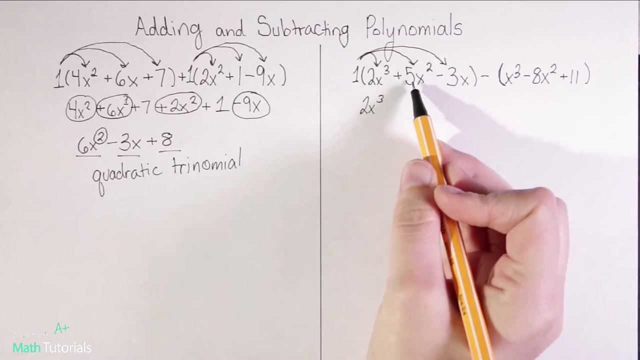 we also would have a 1 here. So there's a positive 1 out here that needs to be distributed throughout this whole problem, throughout this whole parenthesis, to get rid of the parenthesis. So we would distribute this 1 to every single part of the problem. So 1 times 2x cubed is 2x cubed Positive. 1 times 5x squared is positive 5x. 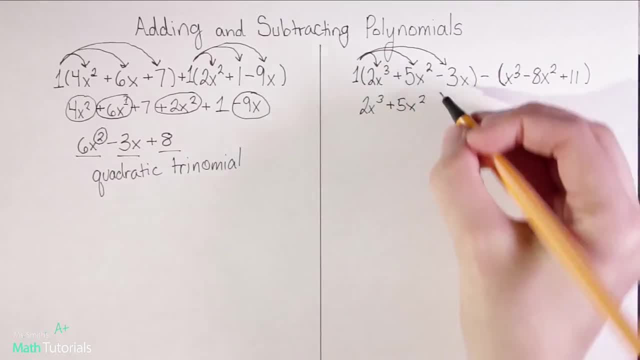 squared And positive 1 times negative. x3 is just negative 3x. So now, coming to this second polynomial, In the same way that we had an understood 1 outside of this, we have an understood 1 outside of here, but it's a. 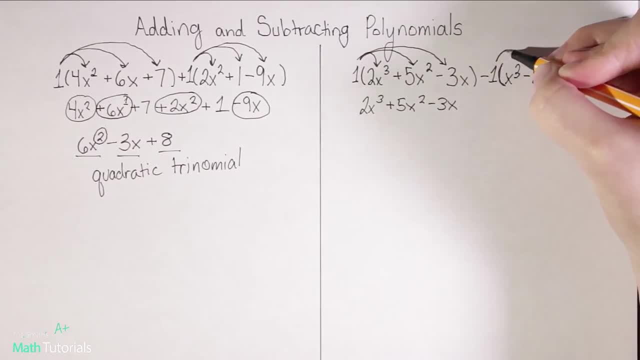 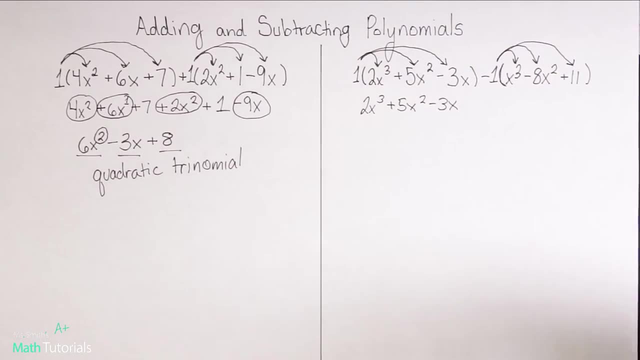 negative 1.. We also need to distribute this negative 1 through this whole polynomial, And the thing about multiplying a negative 1 is that it's going to change the sign of whatever is within the polynomial. So let's see this in action. Negative 1 times positive x3 is now going to give me negative x3.. Negative 1 times negative: 8x. 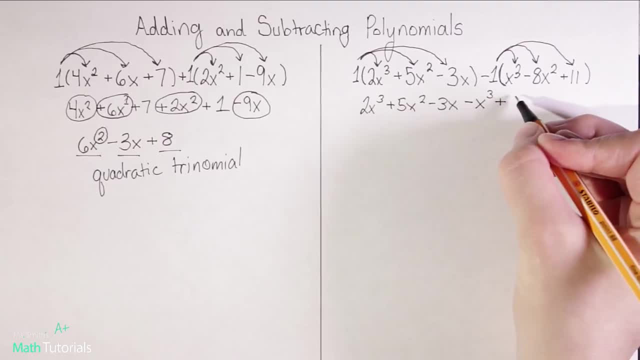 squared is going to give me a negative times a negative is a positive. 8x squared, A negative 1 times a positive 11 is going to give me a negative 11.. So that's why I really like to show this step, even when it's positive, because it's happening, whether it's positive or 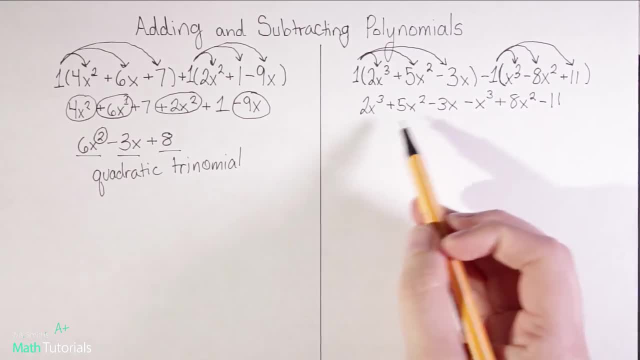 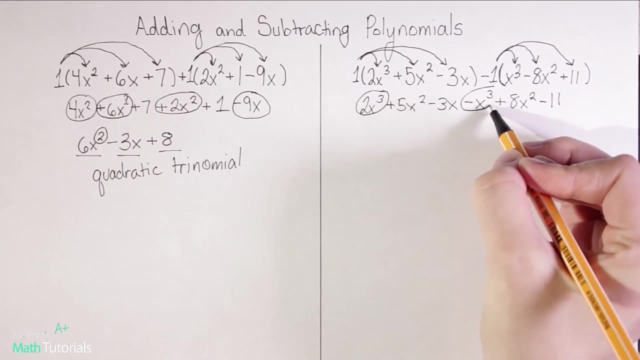 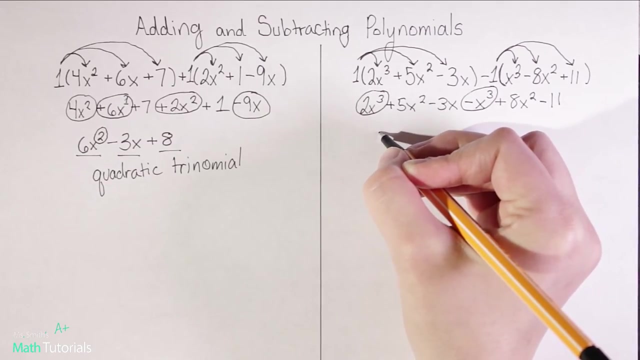 negative. so now that we've gotten all that out of the way, let's combine our like terms. looking through here, I've got a 2x cubed and a negative x cubed that I can go ahead and combine. so 2 minus 1 would be just 1, so it would just be x. 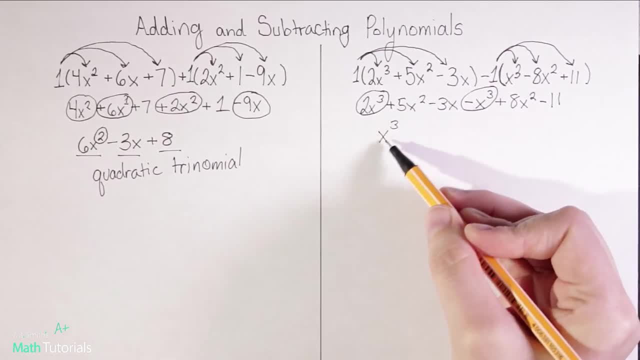 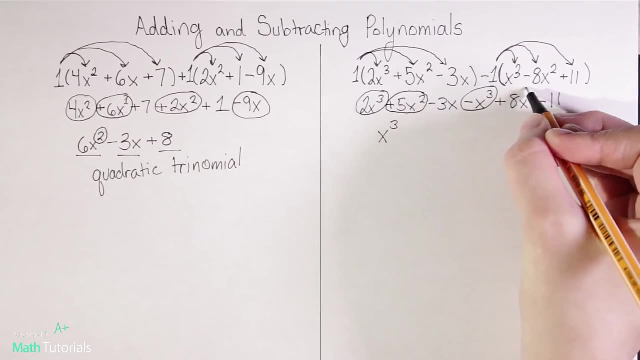 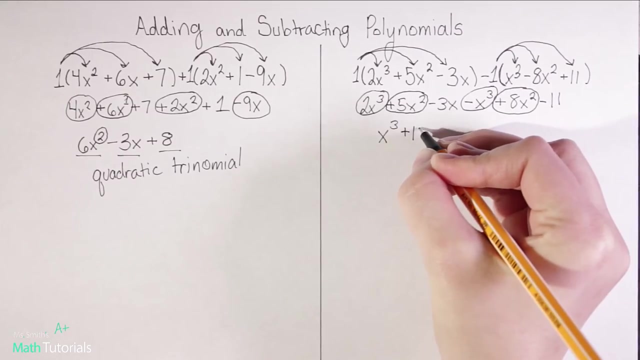 cubed, because remember, our variable and exponent stay the exact same when we're adding or subtracting. next, I've got a positive 5x squared and a positive 8x squared. I can combine. so 5 plus 8 is a positive 13, and then it would stay x. 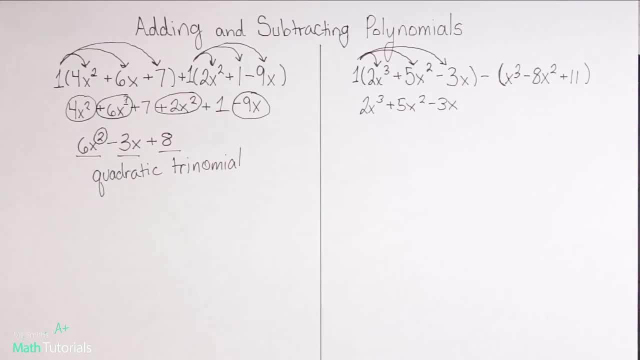 x three is just negative three x. So now, coming to this second polynomial, in the same way that we hadn't understood one outside of this, We haven't understood one outside of here, but it's a negative one- We also need to distribute this negative one through this whole pie. 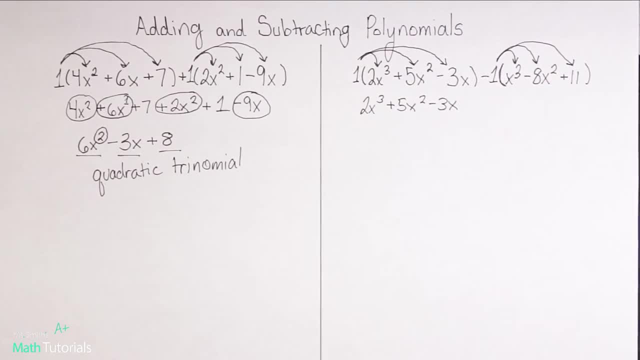 polynomial, And the thing about multiplying a negative 1 is that it's going to change the sign of whatever is within the polynomial. So let's see this in action. Negative 1 times positive x. cubed is now going to give me negative x. 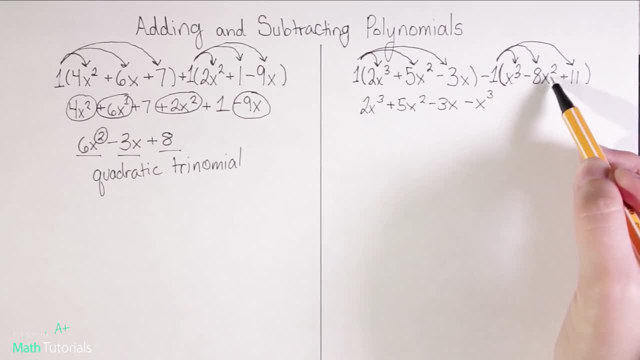 cubed: Negative 1 times negative: 8x squared is going to give me a negative times a negative is a positive 8x squared And negative 1 times a positive 11 is going to give me a negative 11.. So that's why I really like to show this. 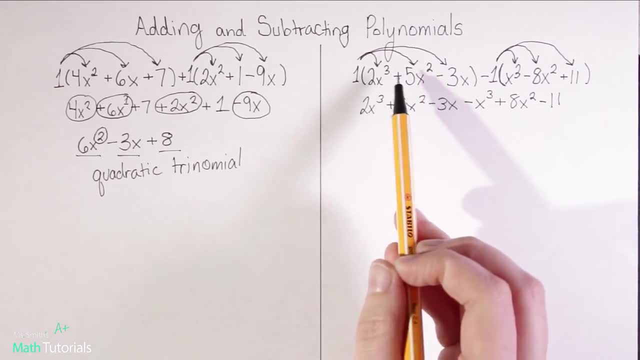 step of distributing the 1 even when it's positive, because it's happening whether it's positive or negative. So now that we've gotten all that out of the way, let's combine our like terms. Looking through here, I've got a 2x cubed and a 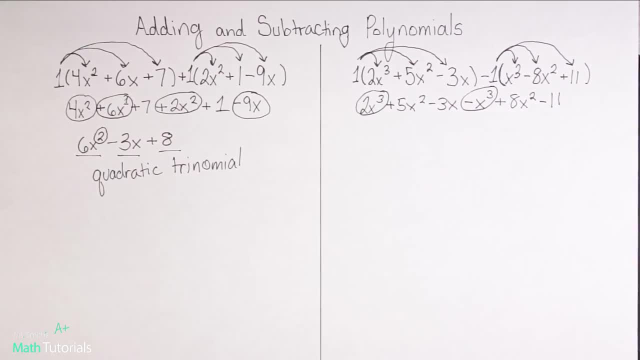 negative x cubed, that I can go ahead and combine. So 2 minus 1 would be just 1.. So it would just be x cubed, because, remember, our variable and exponent stay the exact same when we're adding or subtracting. Next, I've got a positive 5x squared and a positive 8x squared. I can combine, So 5. 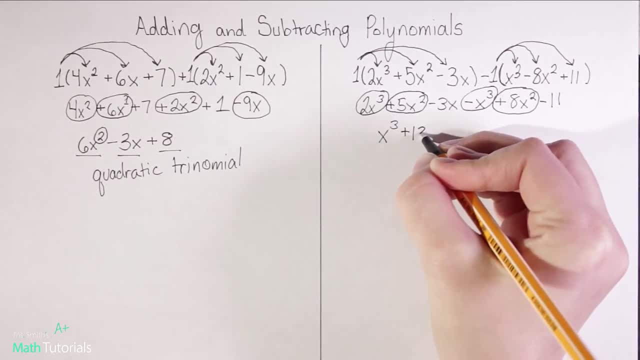 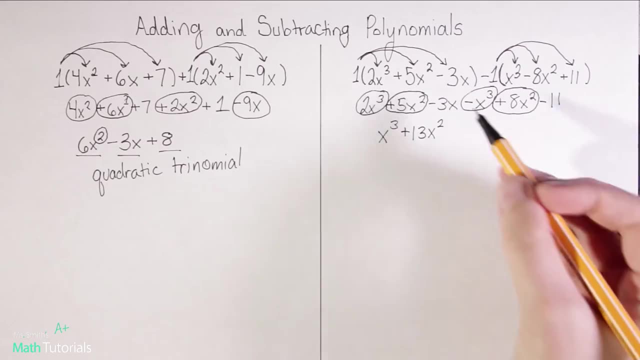 plus 8 is a positive 13, and then it would stay x squared. Next, I've got just this negative 3x to the first power, and there's nothing to combine that with, so it'll just stay the same. And my constant negative 11. there's nothing to combine that with, so that will just stay the same. So this: 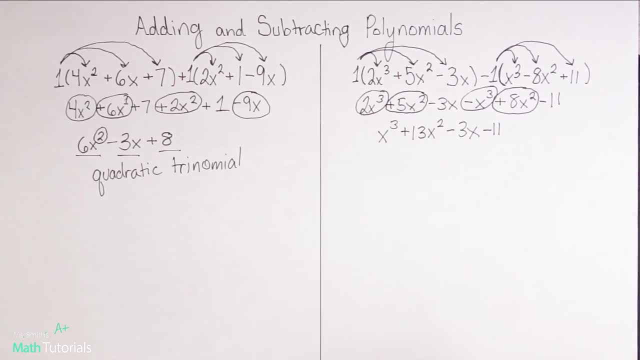 is as low as it can go, because I can't combine these terms any further. So I'm going to go ahead again, just for fun, just for review, I'm going to name this polynomial- So I'm going to give it a first name- based on its degree, In this case my highest exponent, my degree, is 3.. We call that.